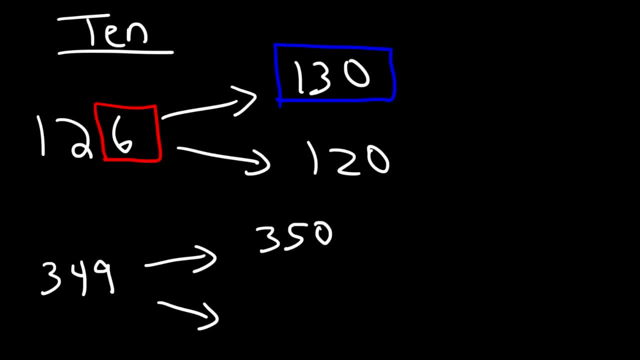 4 or change it to a 5.. So it's either going to be 350 or 340 if we're going to round it to the nearest 10.. So which one is it going to be? Well, looking at the 9,, this is in the. 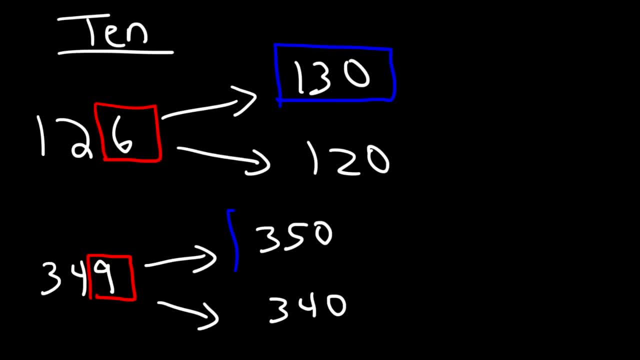 category of 5.. So we're going to keep the 4 or change it to a 5.. So it's either going to be a 5 or more, So therefore we need to round it up to 350.. Let's try one more example. 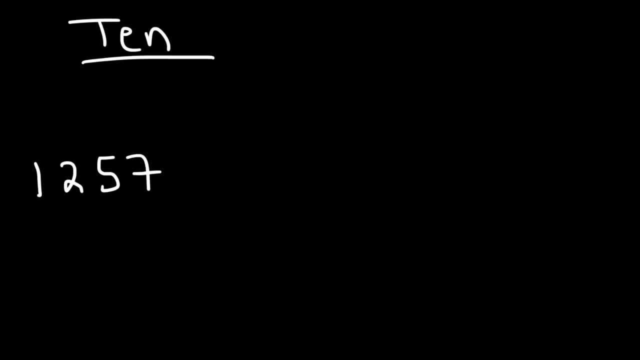 So round this number to the nearest 10.. So this is the tens place. We're either going to keep it a 5 or a 6. And this we need to make it a 0. So it's either going to be 1260. 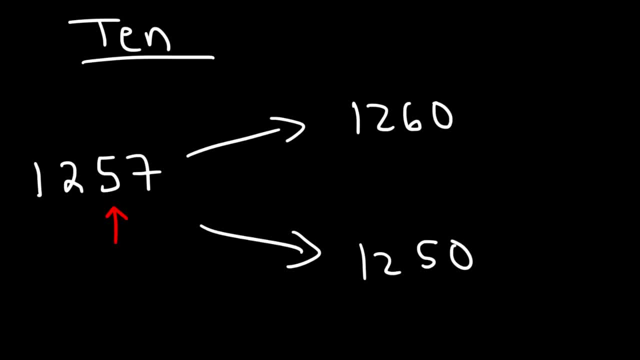 or it's going to be 1250.. So we need to look at the next number. So it's either going to be a 5 or a 6.. So this is in the category of 5 or more. So we need to round up to 1260.. 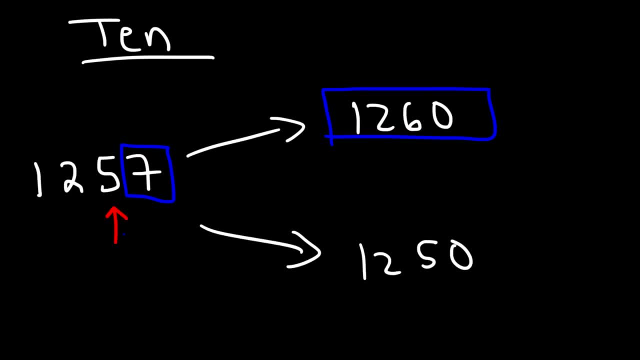 And so that's how you can round to the nearest 10.. But what if we wanted to round to the nearest 100? What should we do? So let's start with an example. Let's say that we have 369.. Round it to the nearest 100.. So this is the ones digit, This is the tens digit, This is. 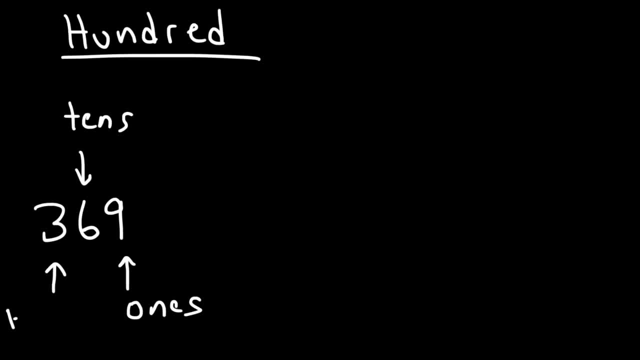 the tens digit And here is the hundreds digit. So we need to either keep it a 3 or we need to round up to a 4.. And everything after that will be a 0. So these two numbers, we're going to convert them into zeros. So either we round it up to 400 or we round it. 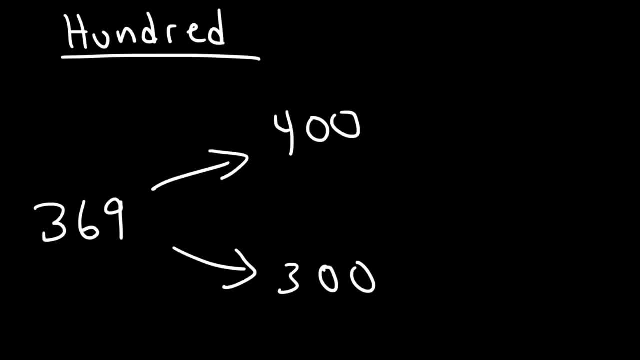 down to 300 if we're going to round it to the nearest 100.. So, looking at the next number, it's a 6.. So that's 5 or more, which means we're going to round up to 400.. Let's try. 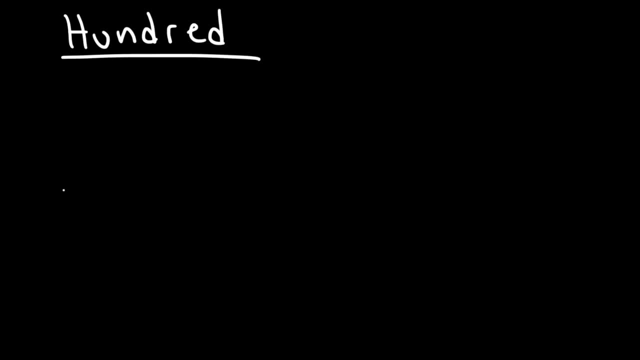 another example. So let's say we have the number 2349.. So this is the hundreds place. So it's either going to go up to a 4, followed by 2 zeros, or it's going to go down to a 3,. 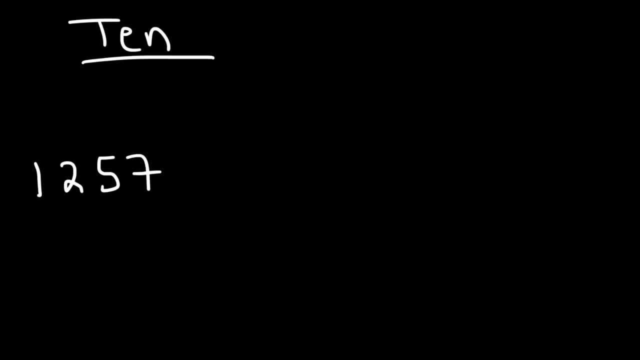 So round this number to the nearest 10.. So this is the tens place. We're either going to keep it a 5 or a 6. And this we need to make it a 0. So it's either going to be 1260. 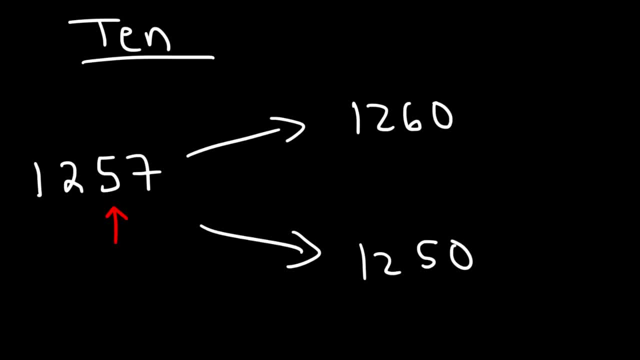 or it's going to be 1250.. So we need to look at the next number. So it's either going to be a 5 or a 6.. So this is in the category of 5 or more. So we need to round up to 1260.. 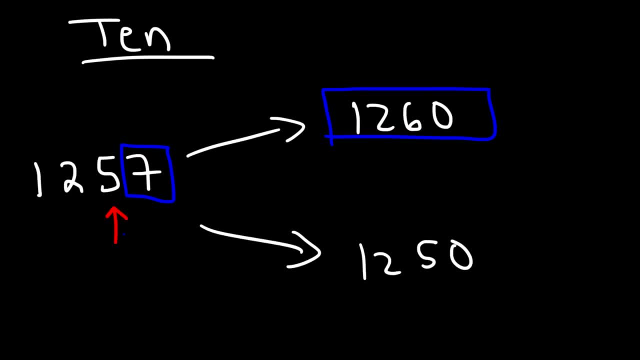 And so that's how you can round to the nearest 10.. But what if we wanted to round to the nearest 100? What should we do? So let's start with an example. Let's say that we have 369.. Round it to the nearest 100.. So this is the ones digit, This is the tens digit, This is. 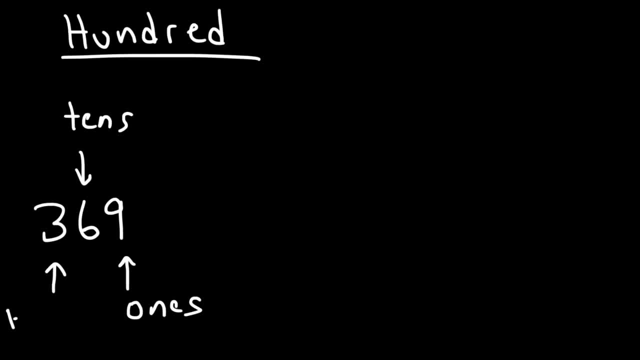 the tens digit And here is the hundreds digit. So we need to either keep it a 3 or we need to round up to a 4.. And everything after that will be a 0. So these two numbers, we're going to convert them into zeros. So either we round it up to 400 or we round it. 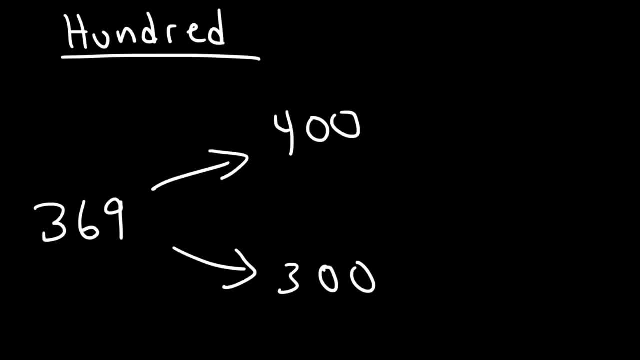 down to 300 if we're going to round it to the nearest 100.. So, looking at the next number, it's a 6.. So that's 5 or more, which means we're going to round up to 400.. Let's try. 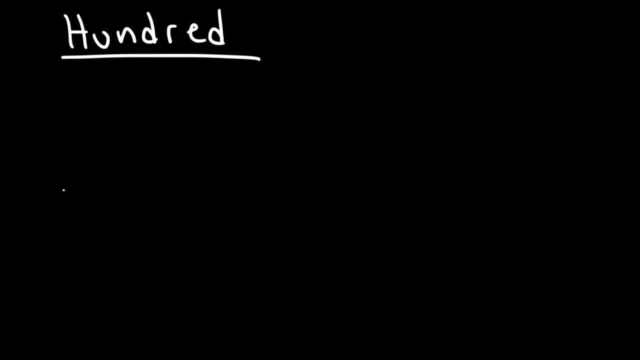 another example. So let's say we have the number 2349.. So this is the hundreds place. So it's either going to go up to a 4 followed by two zeros, or it's going to go down to a 4 followed by two zeros. So, looking at the next number, this is 4 or less. So we're going. 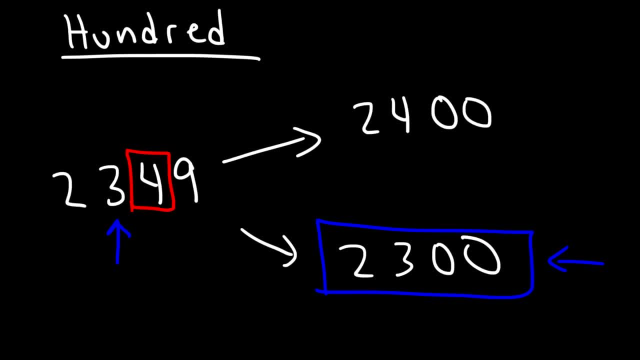 to round it down to 2300. And that's the answer. For the sake of practice, try these two examples: 4258 and let's say 13,526.. So round these two numbers to the nearest 100.. So this is. 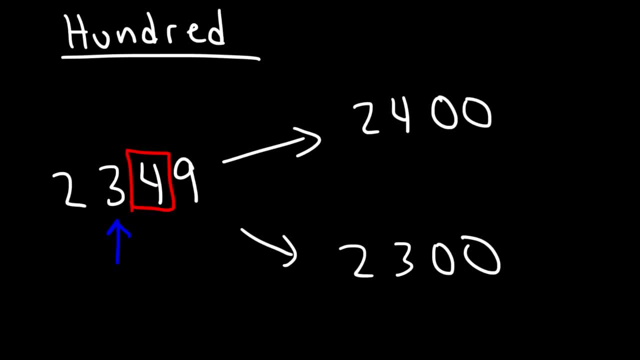 two zeros. so, looking at the next number, this is four or less. so we're going to round it down to 2300 and that's the answer. for the sake of practice, try these two examples: 4258- let's say 13,500- and 26, so around these two numbers to. 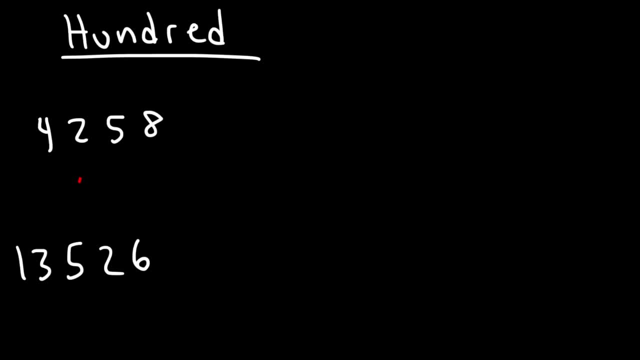 the nearest hundred. so this is the hundreds place we need to, either rounded up to a three followed by two zeros, or rounded down to a two followed by two zeros. so, looking at the next number, it's five or more, which means we're going to round it up to 4300. now for the next example. the five is in the hundreds. 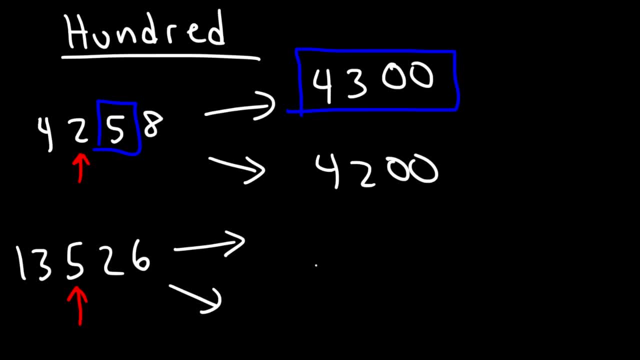 place. so we either round it down by keeping it a five followed by two zeros, or rounded up by keeping it a six followed by two zeros. so the next number is a two. so that's four or less, which means we're going to round it down to 13,500. and that's it for rounding to the. 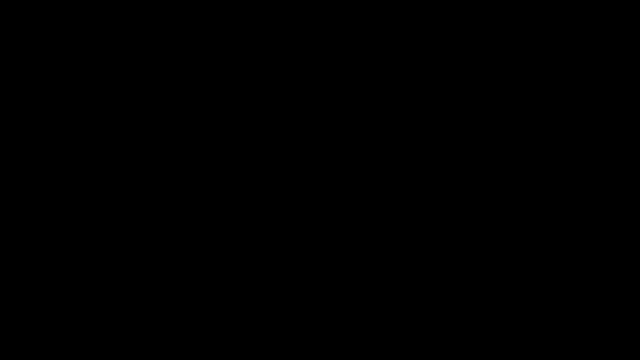 nearest hundred. now for the next example. let's talk about how to round it to the nearest tenth. so let's say, if we have the number 5.367, round it to the nearest tenth. so we know this is the ones digit and this here is the tenths digit and this is the hundreds digit. so 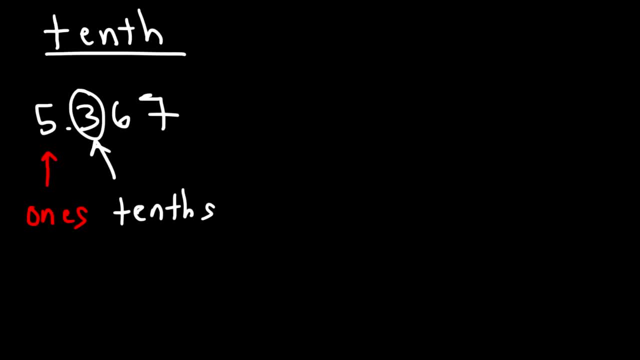 we're going to round it to the tenths digit, so either that's going to go up to 5.4 or down to 5.3. becomes a zero, so we don't have to say 5.300, that's the same as 5.3. so looking: 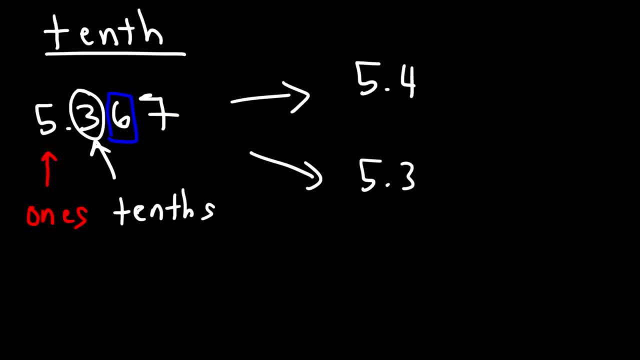 at the next number, which is a six. that's in the category of five or more. so we need to round it up to 5.4. so let's try another example. so let's say we have the number 12.342, round it to the nearest tenth. 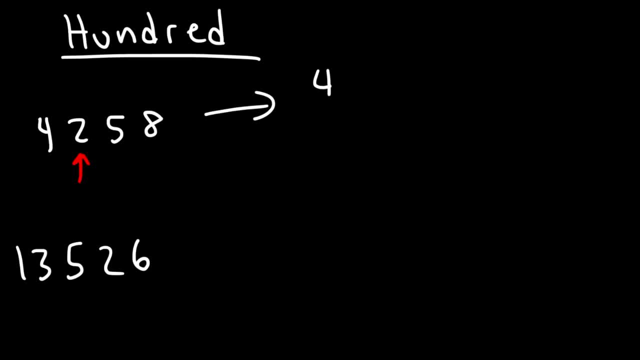 the hundreds place. So we either round it up to a 3 followed by two zeros, or round it down to a 2 followed by two zeros. So looking at the next number, it's 5 or more, which means we're going to. 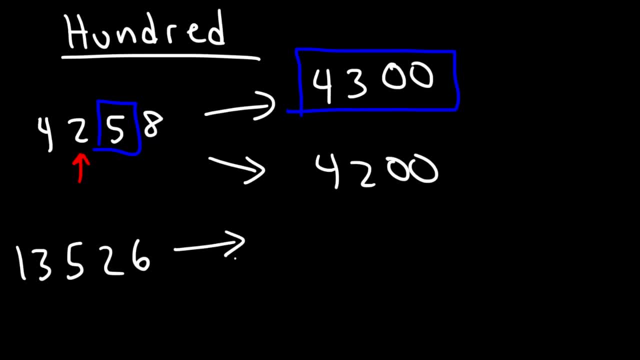 round it up to 4300.. Now for the next example. the 5 is in the hundreds place, So we either round it down by keeping it a 5 followed by two zeros, or round it up by keeping it a 6 followed by two zeros. So the next number is a 2.. So that's 4 or less, which means we're. 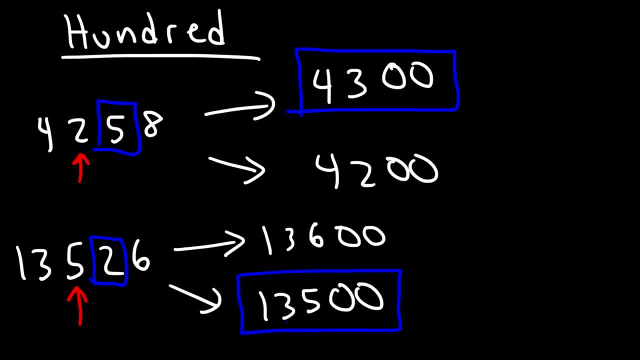 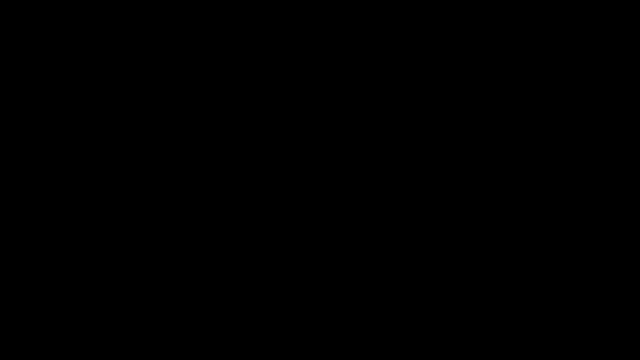 going to round it down to 13,500.. And that's it for rounding to the nearest 100.. Now for the next example. let's talk about how to round it to the nearest tenth. So let's say, if we have the number 5.367.. 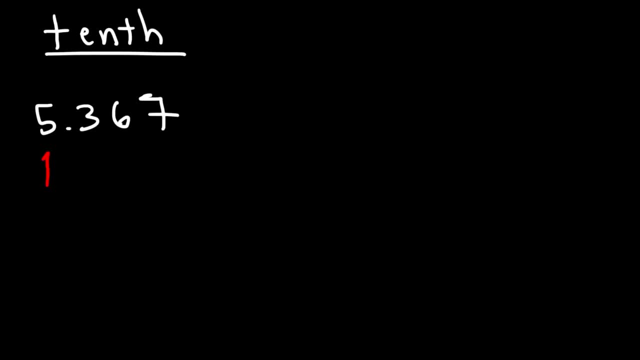 The nearest tenth. So we know this is the ones digit And this here is the tenths digit And this is the hundredths digit. So we're going to round it to the tenths digit. So either that's going to go up to 5.4 or down to 5.3.. Every other number becomes a zero. 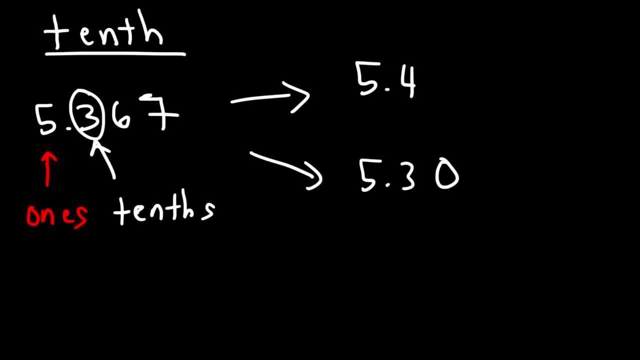 So we don't have to say 5.300.. That's the same as 5.3.. So looking at the next number, which is a 6,, that's in the category of 5 or more. So we need to round it up to 5.4.. So let's try another example. So let's say we: 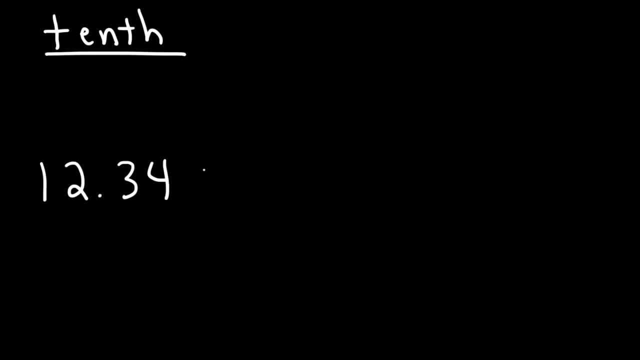 have the number 12.342.. Round it to the nearest tenth, So here is the tenths digit. So we're either going to keep it 12.3 or make it go up to 12.4.. So looking at the next number, 4, it's less than 5, which means that we're going to round it down to 12.3.. 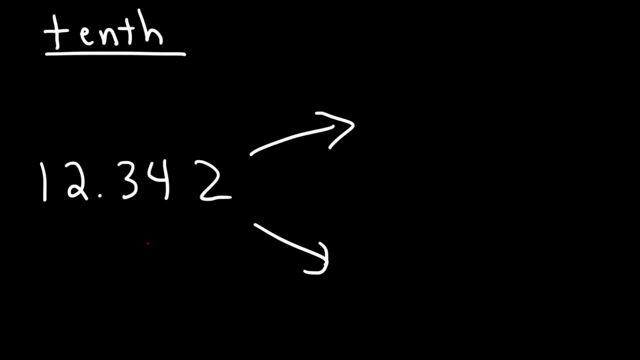 so here is the tenths digit. so we're either going to keep it 12.3 or make it go up to 12.4. so, looking at the next number four, it's less than five, which means that we're going to round it down to 12.3. now go ahead and try these two. 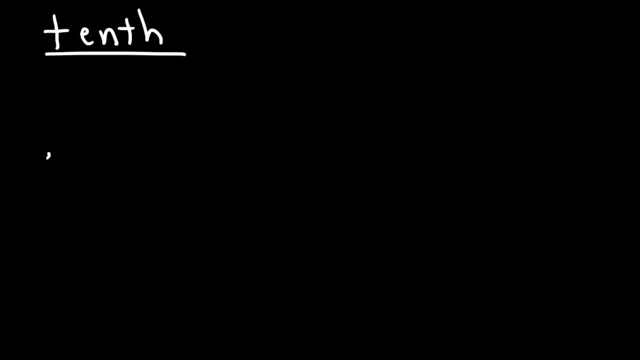 examples. so let's say eight point one, four, seven, six and one. thirty two point three, five, nine, one. so let's identify the tenths place. so either we're going to keep it at 8.1 or rounded up to 8.2. looking at the next number, it's four or less. so we're going. 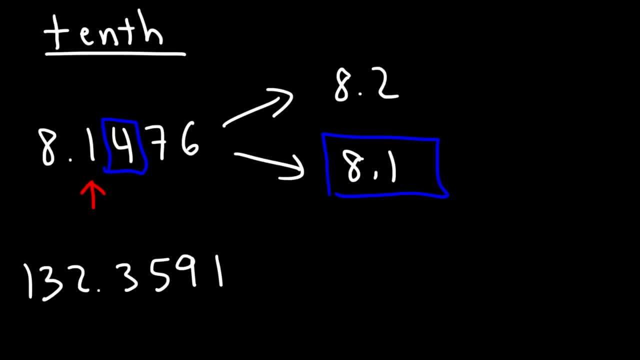 to run it down to 8.1. for the next example, three is in a tenths place, so we're either going to keep it down at 3, that is, 132.3, or round it up to 132.4.. So the next number is a 5, so since it's 5 or more, we need to round up to 132.4.. 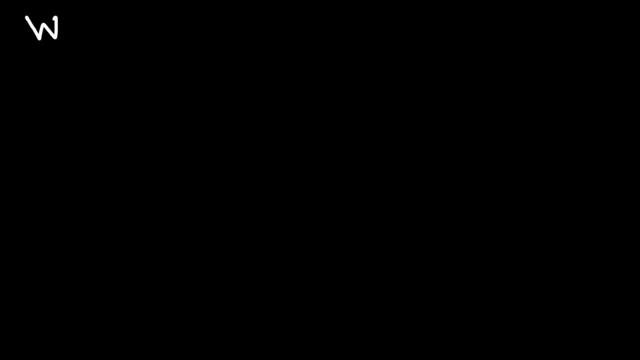 Now, in the next example, we're going to focus on rounding to the nearest whole number. If you get a problem like this, it's the same as rounding it to the ones digit. So let's say, if we have the number 34.235,, what's the answer? So here is the ones digit. It's either going to go down to 34 or it's. 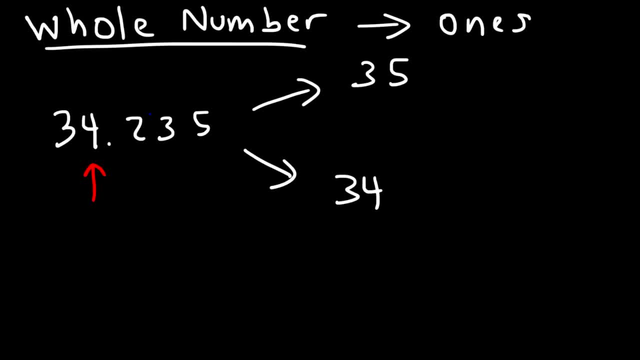 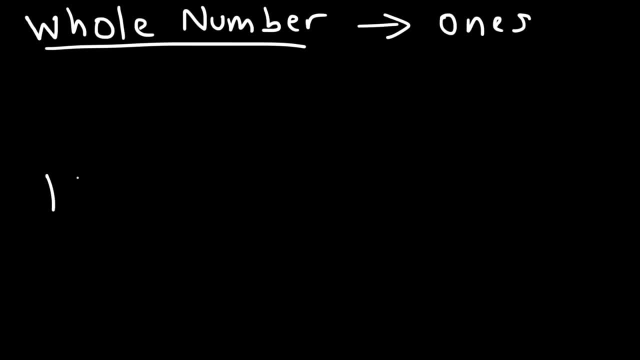 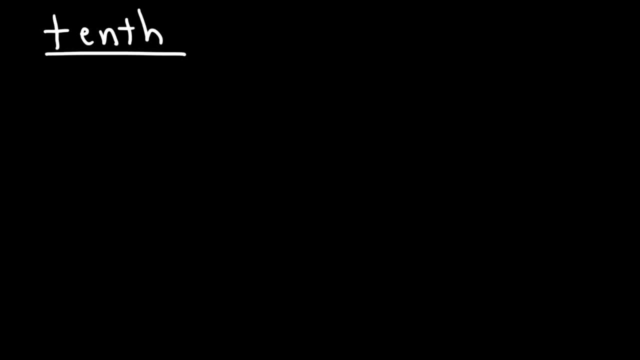 Now go ahead and try these two examples. So let's say 8.1476 and 132.3591.. So let's identify the tenths place. So either we're going to keep it at 8.1 or round it up to 8.2.. 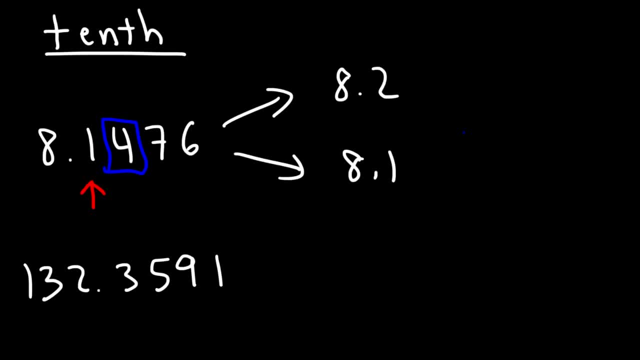 Looking at the next number, it's 4 or less, so we're going to round it down to 8.1.. For the next example, 3 is in the tenths place, so we're either going to keep it down at 3,, that is, 132.3, or round it up to 132.4.. 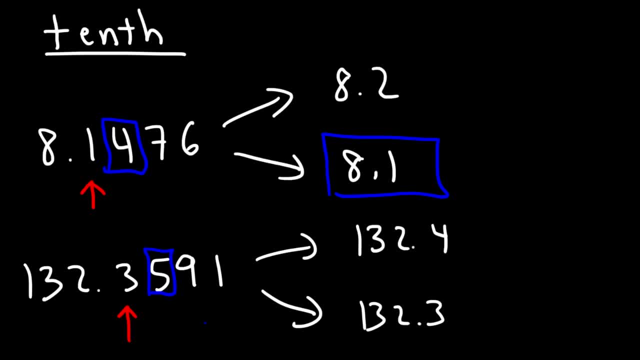 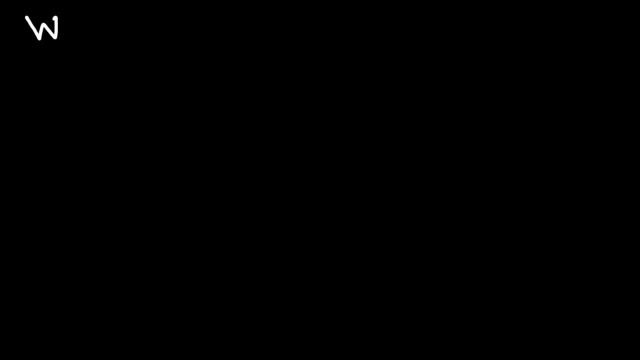 So the next number is a 5, so since it's 5 or more, we need to round up to 132.4.. Now, in the next example, we're going to focus on rounding to the nearest whole number. If you get a problem like this, it's the same. 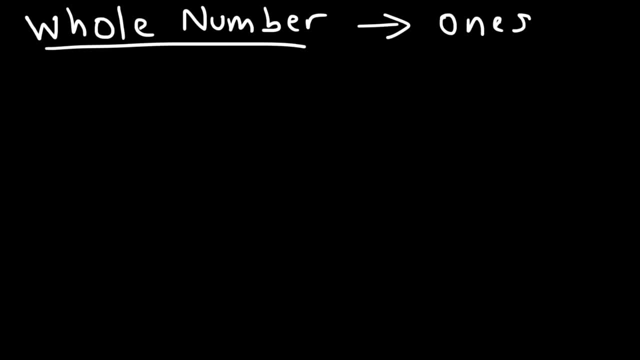 Let's round it to the ones digit. So let's say, if we have the number 34.235,, what's the answer? So here is the ones digit. It's either going to go down to 34 or it's going to go up to 35.. 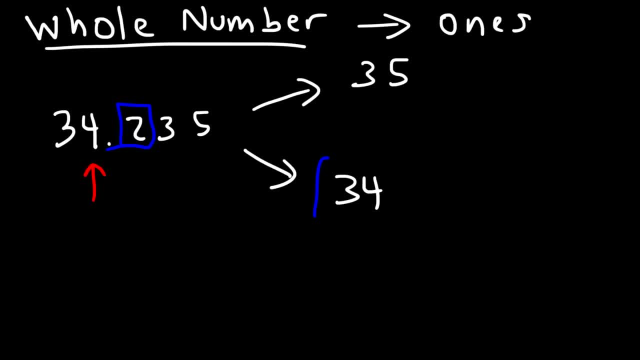 So, looking at the next number, 2, that's less than 5, so we're going to round down to 34.. Now let's consider another example. Let's say if we have 146.581, and round it to the nearest whole number. 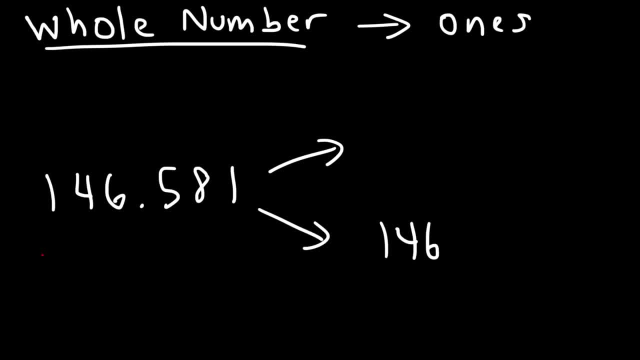 So it's either going to be 146, because we need to stop at the ones digit, or we're going to go up to 147.. So this number, the next number, is 5 or more, which means we need to round up to 147. 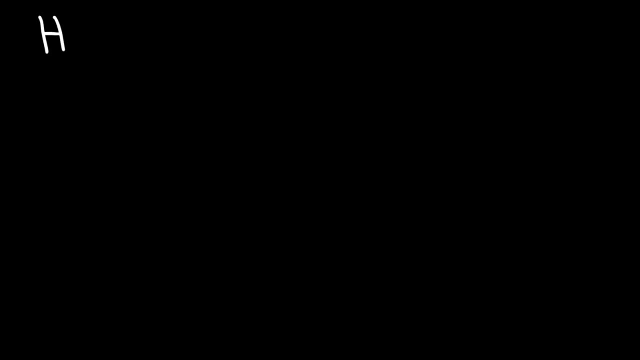 Now let's focus on rounding to the nearest whole number. So let's say, if we have 5.7246, go ahead and round it to the nearest hundredth. So this is the hundredth place. So it's either going to be 5.72, or we're going to round up to 5.73.. 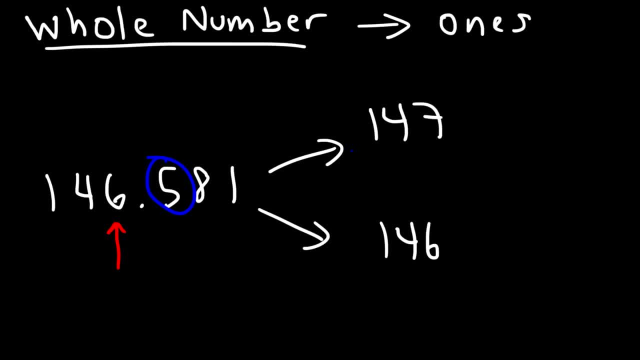 So this number, the next number, is 5 or more, which means we need to round up to 147.. Now let's focus on rounding to. Now let's focus on rounding to the nearest hundredths place. So let's say we have 5.7246. 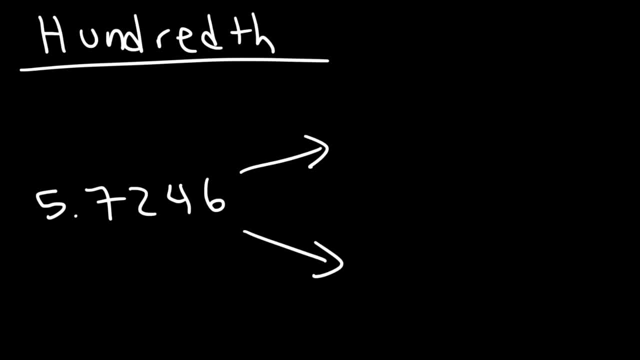 Go ahead and round it to the nearest hundredth. So this is the hundredths place. So it's either going to be 5.72, or we're going to round up to 5.73.. So looking at the next number, 4, that's less than 5.. 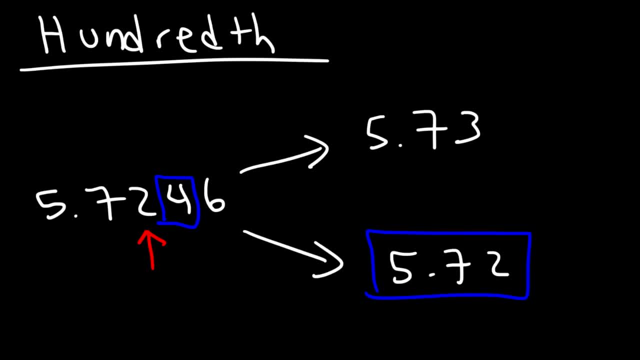 So we need to round down to 5.72.. Now let's say, if we have 14.6899.. So this is the hundredths place. So it's either going to be 14.68, or 14.69.. 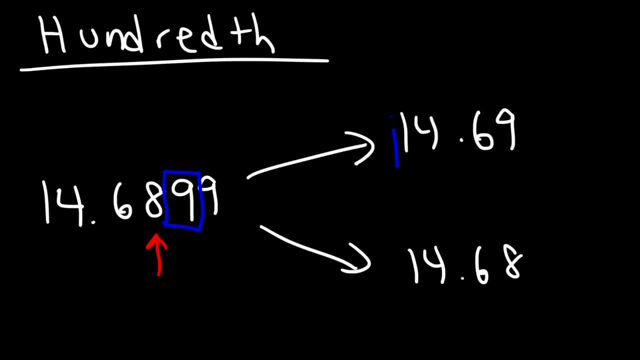 So, looking at the next number, it's greater than 5.. So it's definitely going to round up to 14.69.. Now what if we wanted to round to the thousandth place? So let's say we have the number 3.25614.. 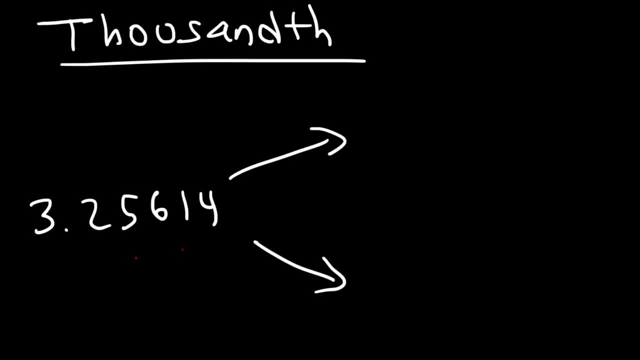 So round it to the nearest thousandth. So this is the thousandth place. We know, this is the tenth, This is the hundredths, And so this has to be the thousandth. So we're either going to keep it at 3.256, or we're going to round it up to 3.257.. 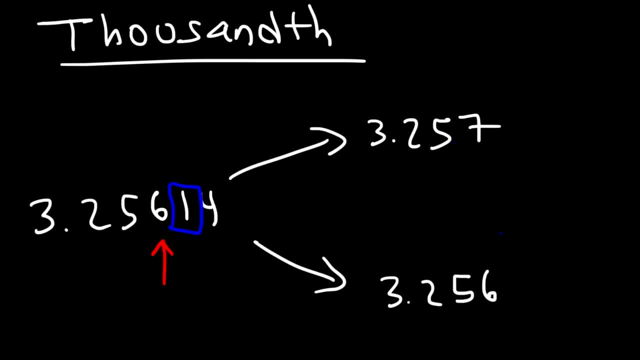 So, looking at the next number, it's less than 5.. So we're going to round it down to 3.256.. Let's work on one more example. So let's say we have 17.87463.. So go ahead and round it up to 3.256.. 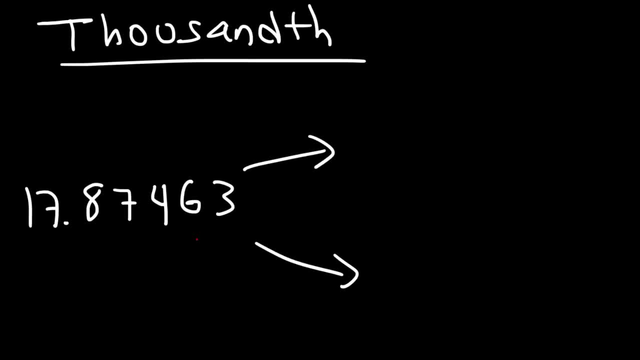 And we're going to round it to the nearest thousandth place. So here is the thousandth digit. So it's either going to be 17.874, or 17.875.. So this is either going to be a 4 or a 5..